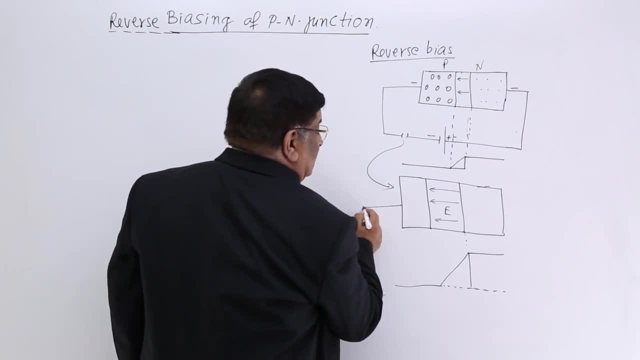 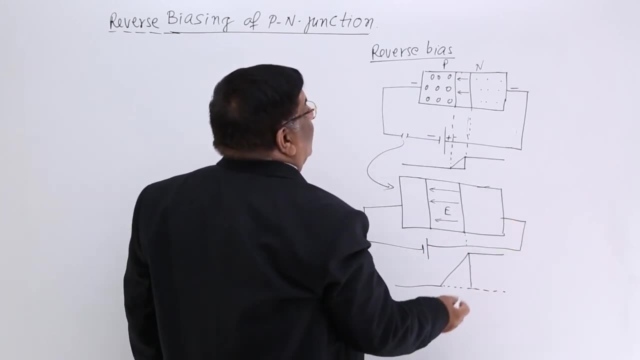 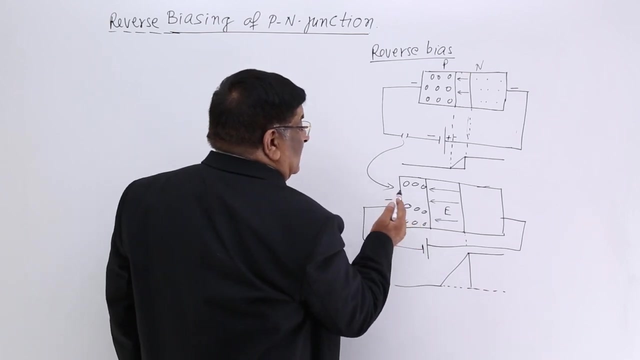 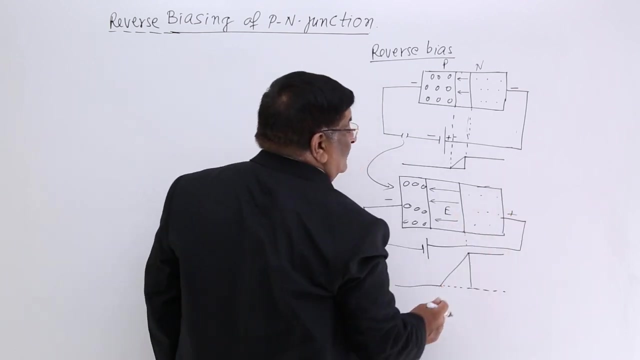 See, what has happened is this is minus and this is plus. here This minus minus will attract positive terminal. Then this n-type terminal will attract negative terminal. So positive plus will attract electron to its sides. If we think in this way, then what? 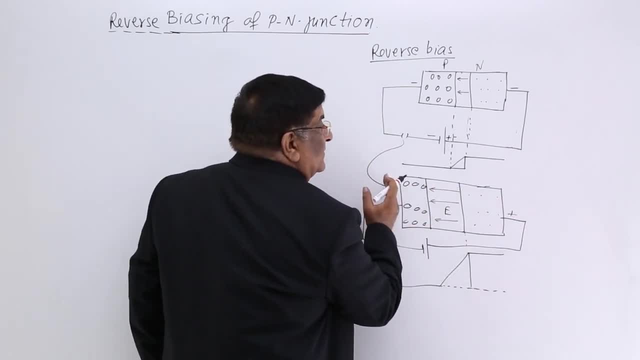 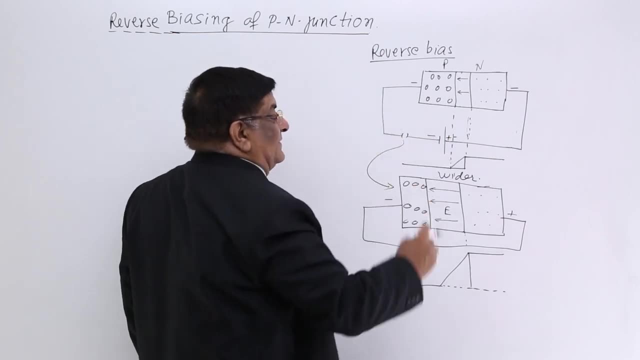 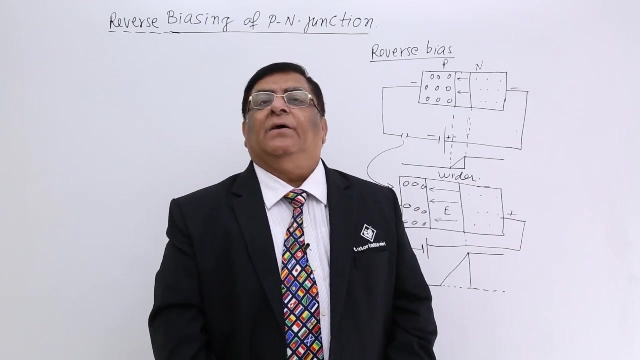 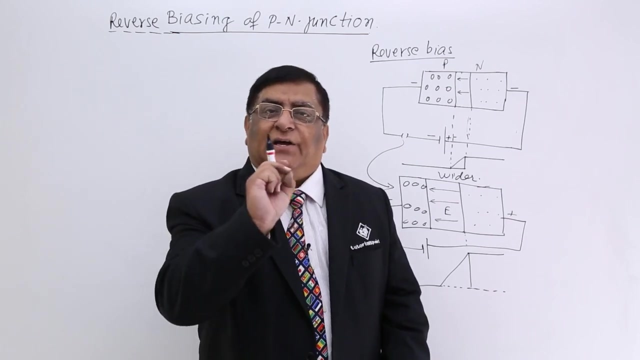 will happen. Electrons move here, positive charges move here and the depletion layer gets wider. So what happens to depletion layer? In reverse bias, it gets wider. Depletion layer represent the resistance, the layer in which there are no charges, no charge carriers. 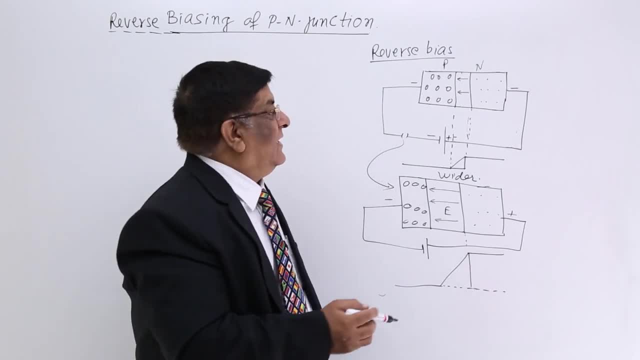 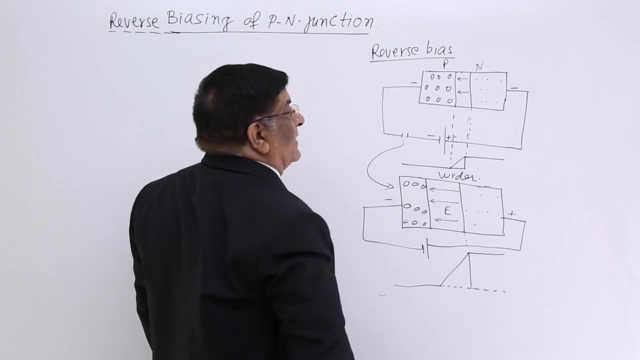 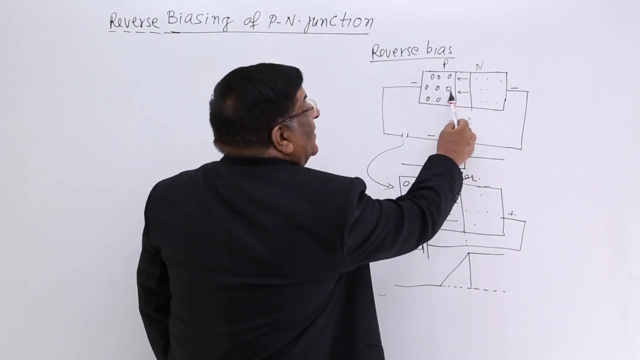 So current cannot pass it. it has to jump through it. And if this has become wider then it is become more difficult for electrons to jump. So the resistance has increased. The resistance has increased. the chances of flowing current have become less. 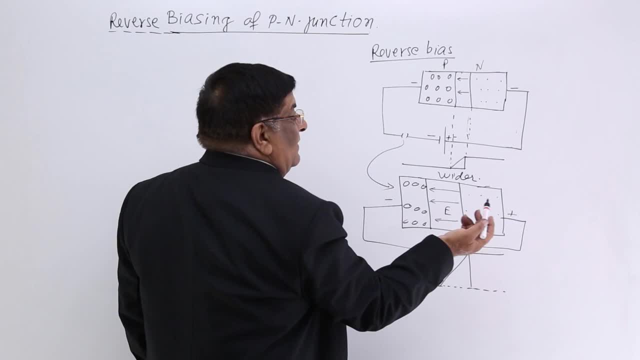 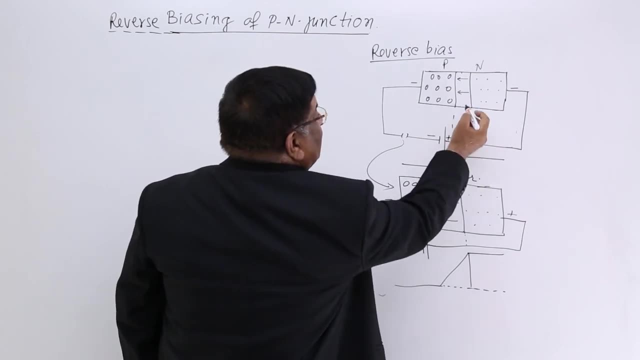 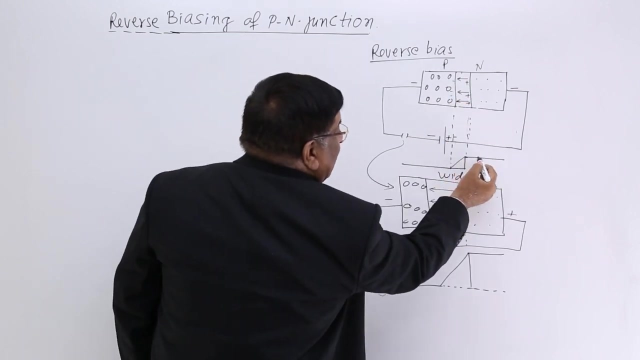 Now, so no current will flow here. Another method of looking to it: There was a potential barrier created here. This is at a higher potential. this is at a lower potential. this is at a higher potential. this is at a lower potential, and there is a difference. This: 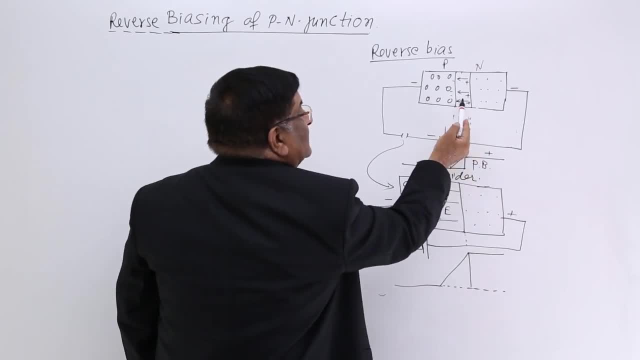 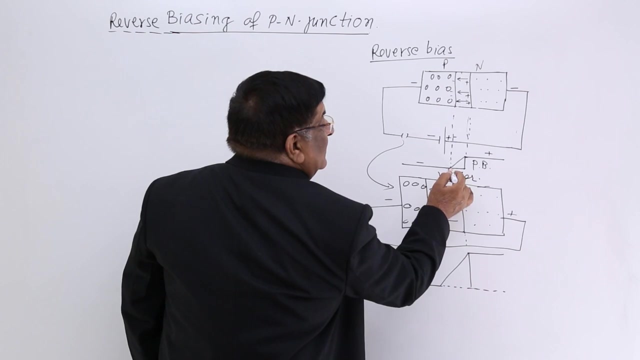 difference is known as potential barrier. Because of this difference, electron cannot jump here. So this is potential barrier and this is electric field. that is potential gradient. If this is the width, then these are the two points and this shows the height of the potential. 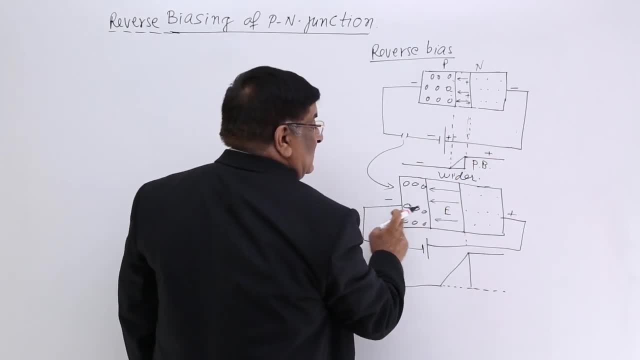 barrier. When this width increase, when this width increase due to this polarity, then what will happen? Same is the gradient, But because this distance is greater, this distance has increased. it is here and it is here Now. this height has increased. That means 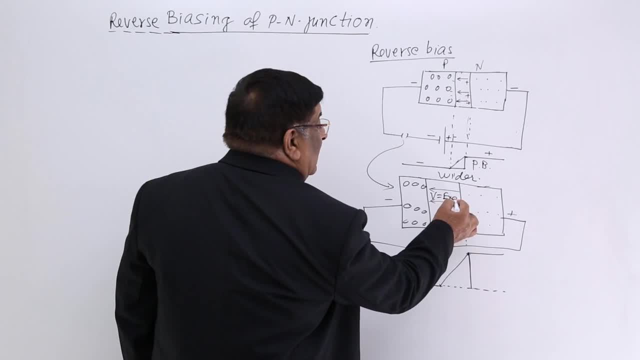 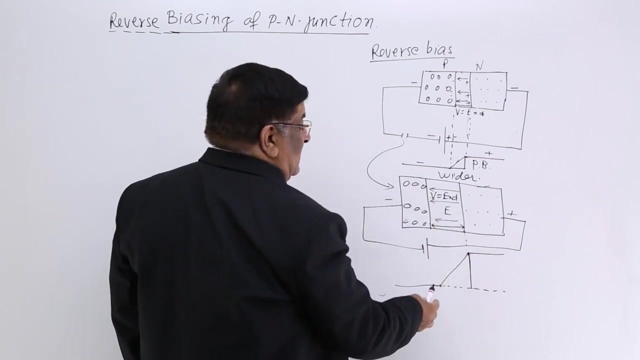 the potential difference. V is equal to E multiplied by D. Here V is equal to E multiplied by D. Here this distance is small, here this distance is large. If the distance is large, then V will increase and that is potential difference as E multiplied by D. So the potential difference, 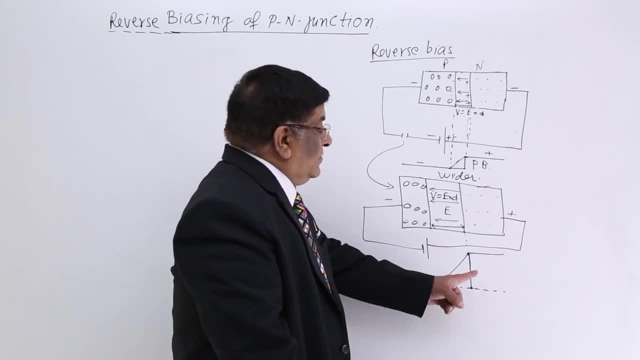 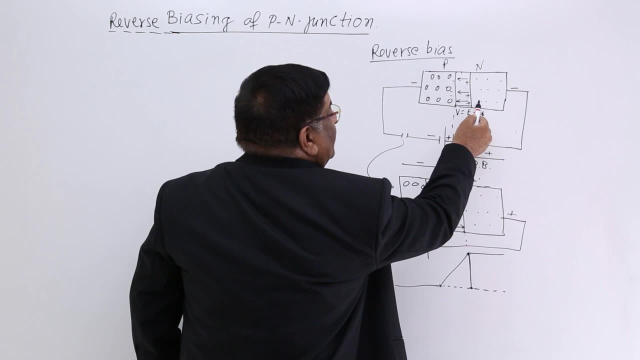 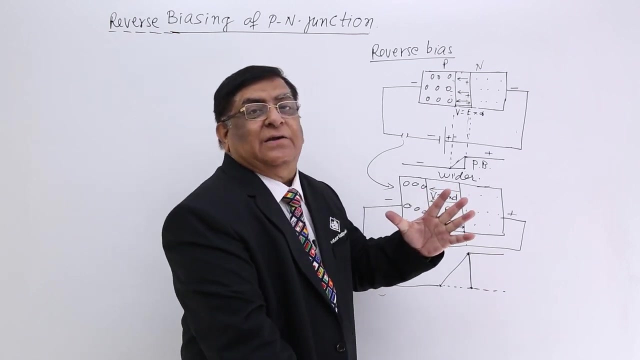 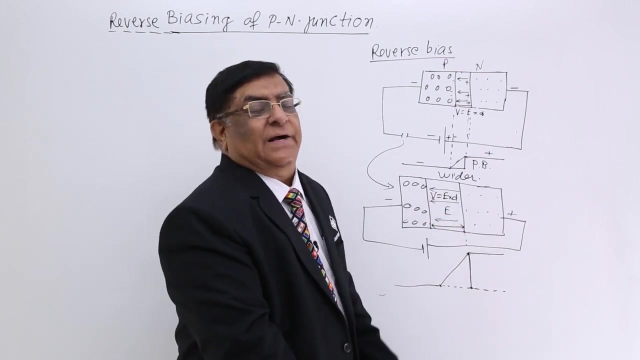 has increased. So this potential difference is potential barrier For this electron. it was little difficult to go here, but for this it is impossible to go here, And impossible to go here, the current cannot flow. Now, if the current cannot flow, it has become a insulator. Again, here is the potential difference, potential barrier. 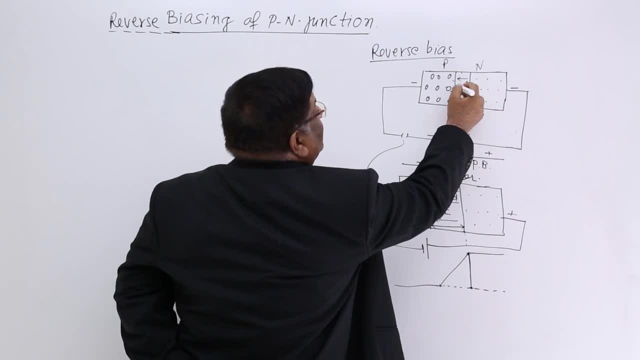 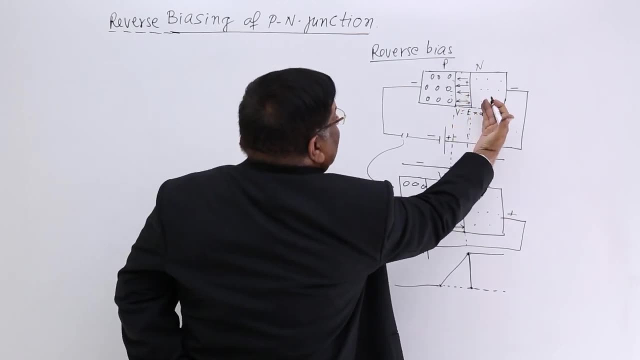 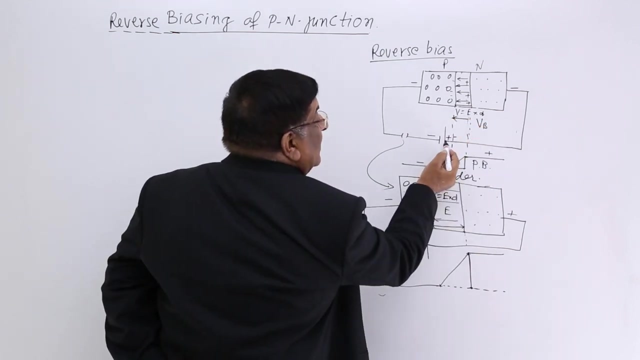 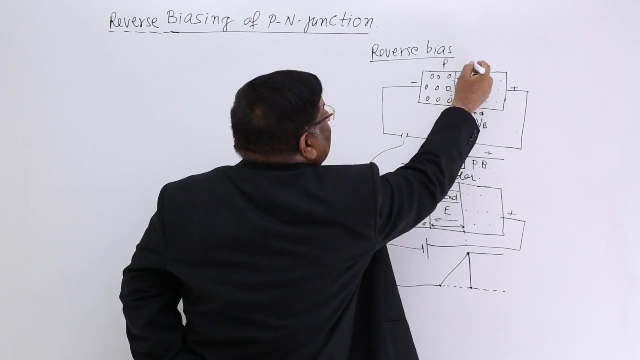 It is a potential barrier created by electric field in the junction. What is its direction? Its direction in this example is here, right to left. This is the direction of V barrier. We have applied a potential difference, plus on this side and minus on this side. So this: 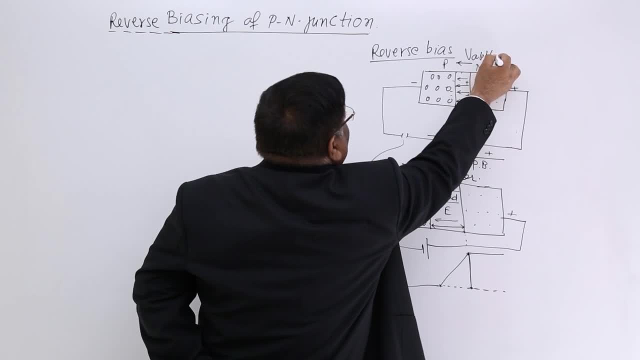 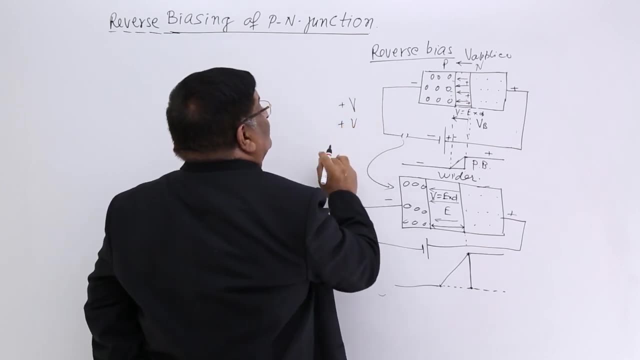 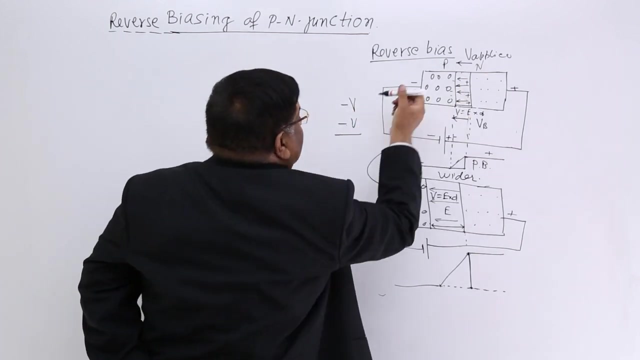 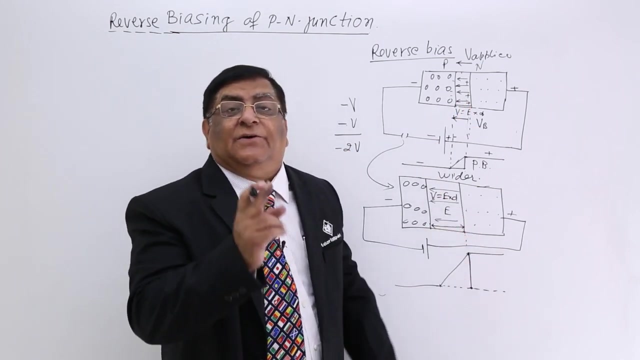 is the direction of V applied. Now you see, both the directions are in the same way. So what will happen? They will get added up, Both are reversed, so we can say Both are same sign, opposite sign. so they get reversed. So the potential barrier has increased In the forward, biasing what was 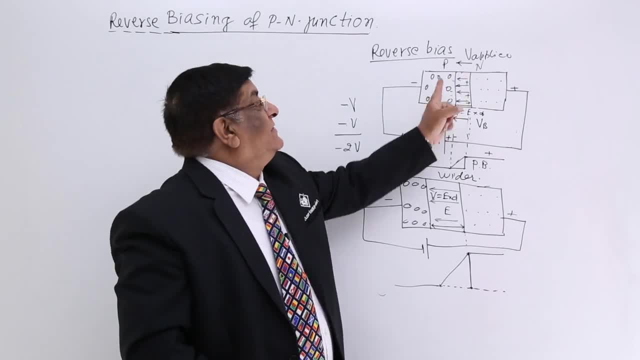 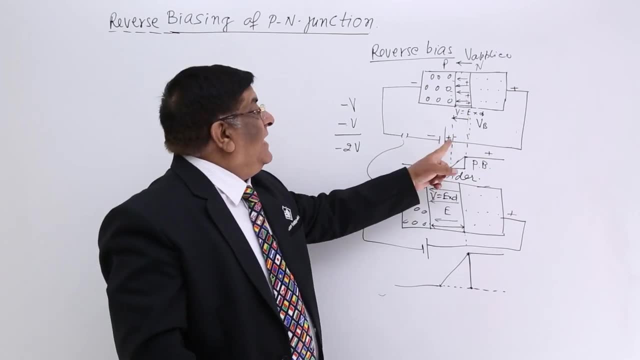 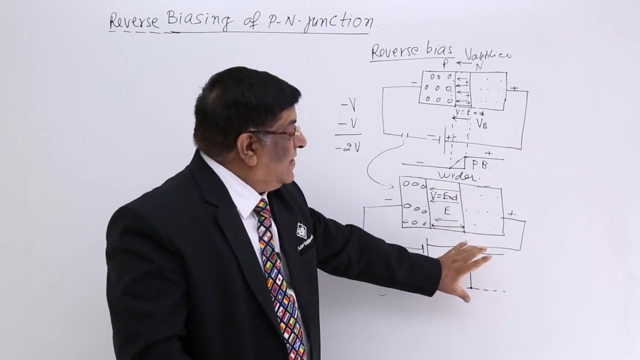 there. This was minus, this was plus. this used to cancel it and it would have become a positive. Then it would have become conductor. here This is the barrier and we have applied in the direction of barrier. So the barrier has become higher. Here it was 1V, now it is 2V. 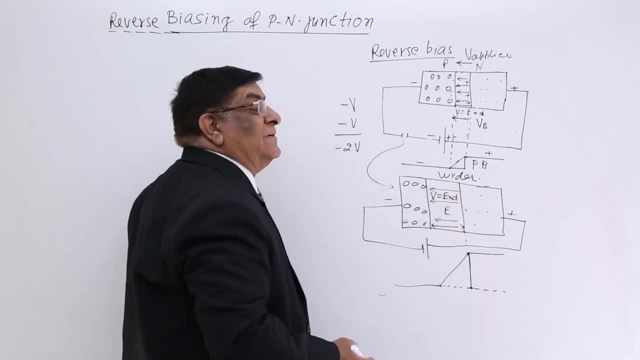 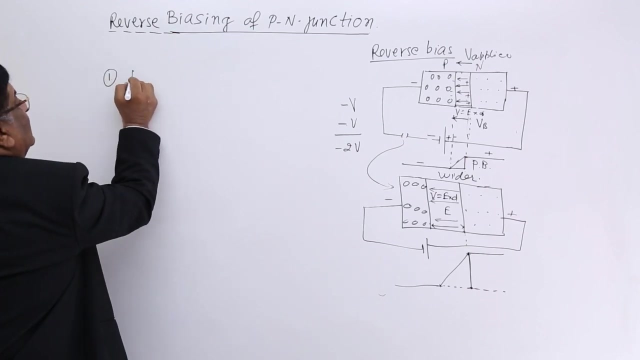 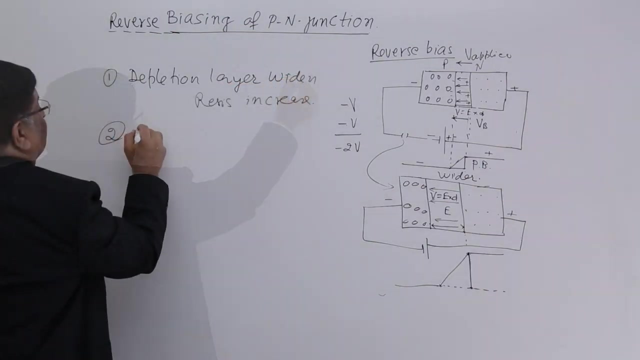 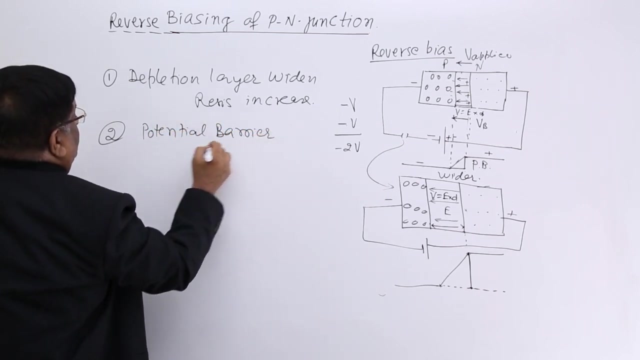 If electron has to go here it has to have double the energy And it does not have so, so it will not go here. So this way potential barrier height has increased. So what are the two effects in reverse biasing Number one? depletion layer widened, So our resistance increase, potential barrier become. 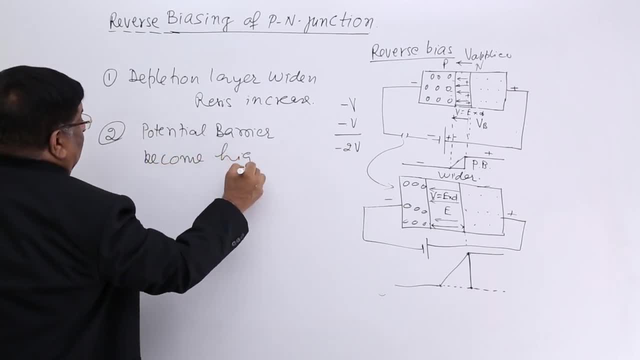 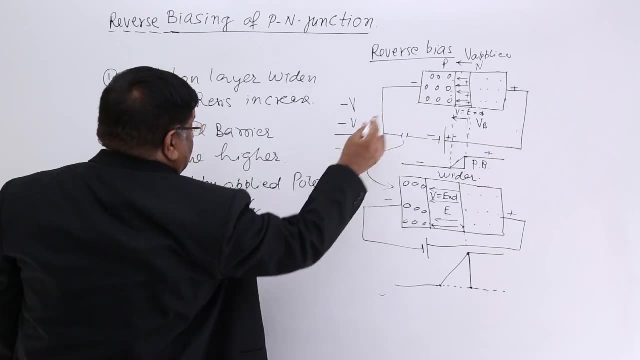 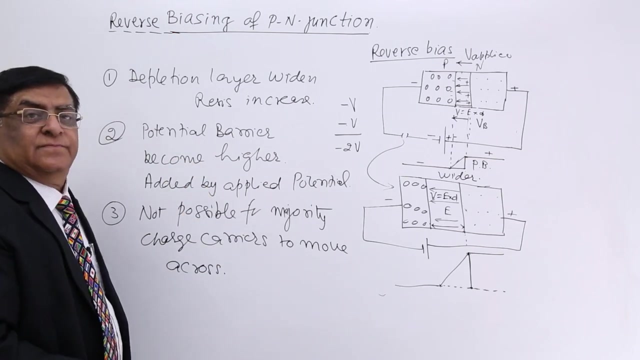 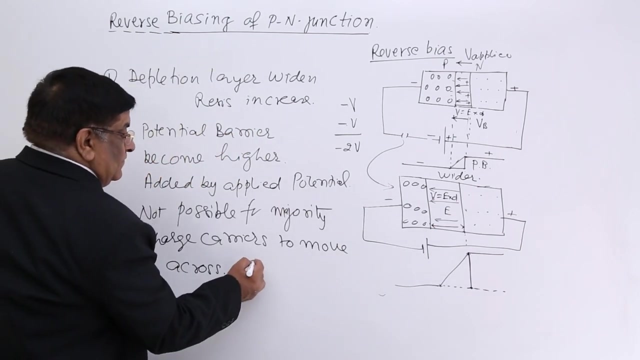 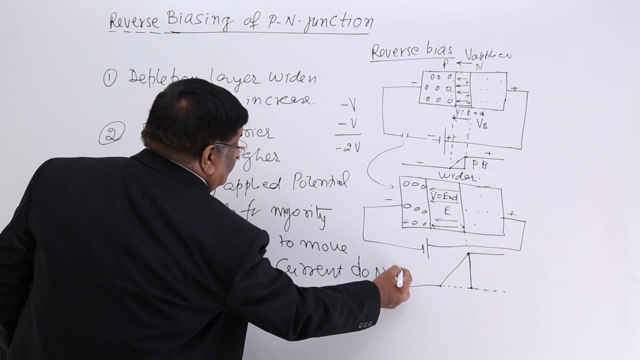 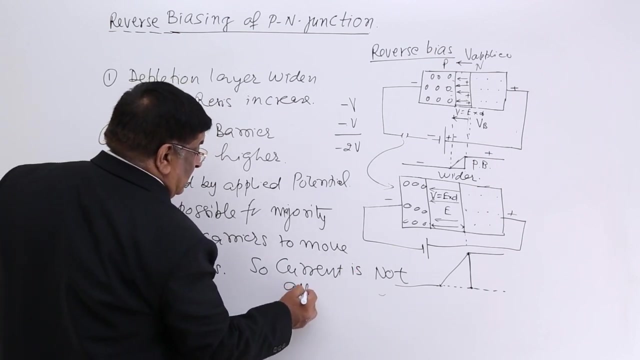 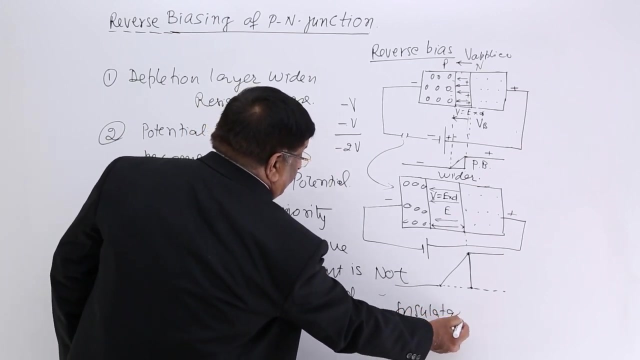 higher Added by applied potential. Not possible for majority charge carriers to move across loss. So they do not move. and if they do not move, what is this? an insulator, So current do not allowed. So current is not allowed. and now what it has become? insulator, So 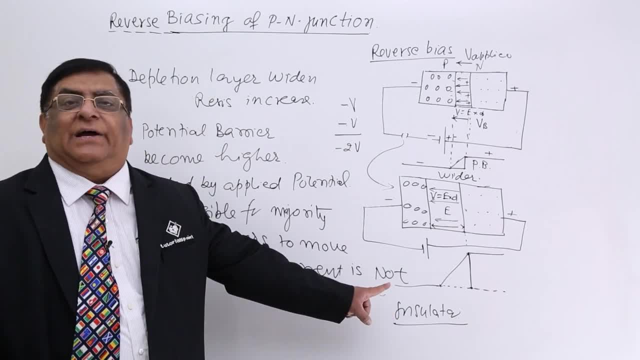 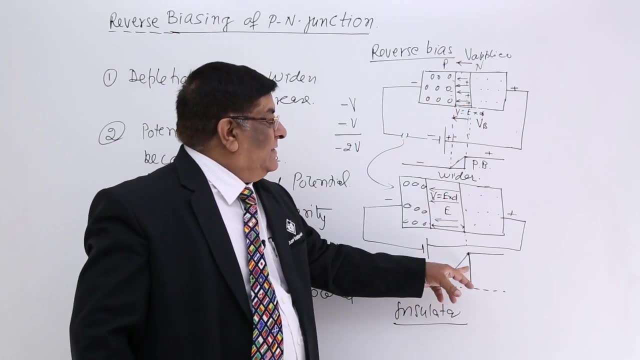 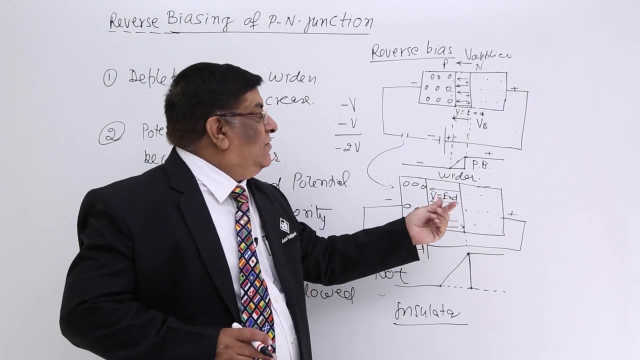 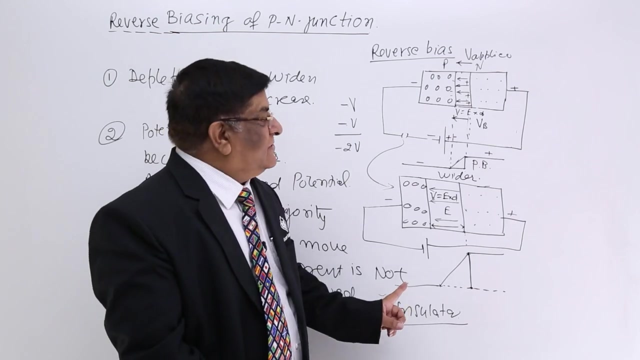 in reverse bias. this act as insulator and the current is not allowed In forward bias. this, the potential barrier, was forward Finished. it had become equal. this layer had shrink to 0 and there was a fast movement of the electric charges. it would have become conductor In reverse barriers. this has increased. 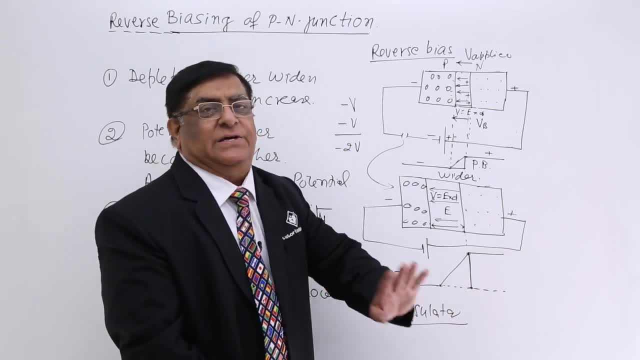 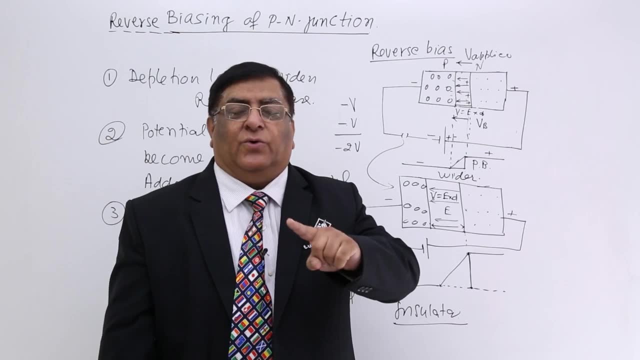 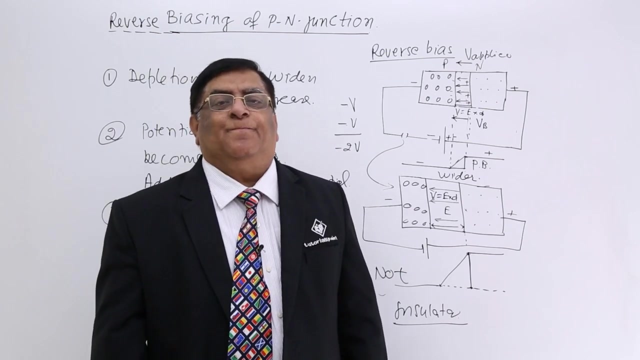 the barrier has become higher and it has become insulator. it will not allow current to flow. You understand this. and now there is another thing that is also very, very important To understand. this phenomena is reverse current. What is reverse current? Reverse current is: 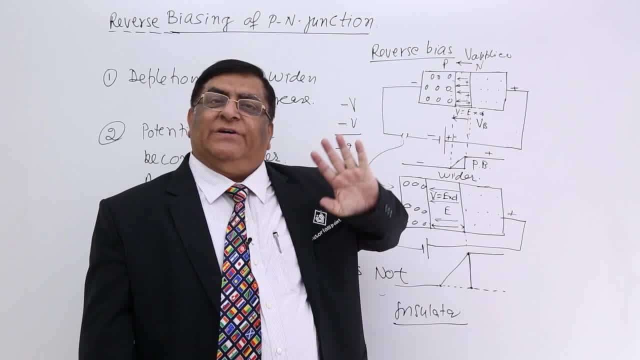 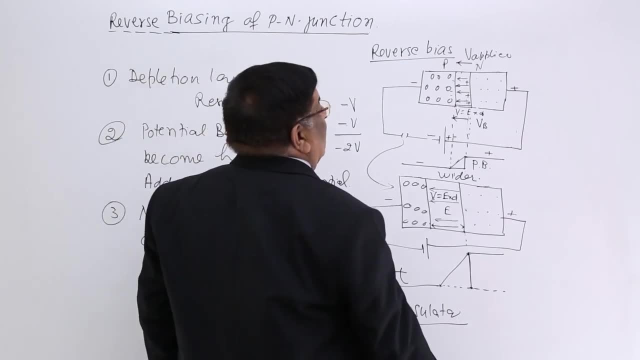 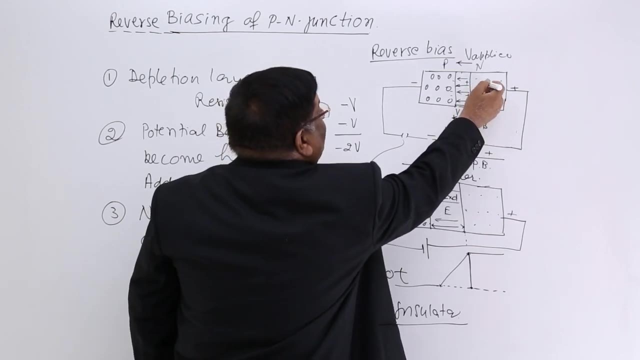 a current flowing in this circuit in reverse biasing only. that is why it is known as reverse current, See in reverse biasing. what is that current? when we say this is a n type semiconductor, the majority charge carriers are electron, but there are certain minority charge carriers. 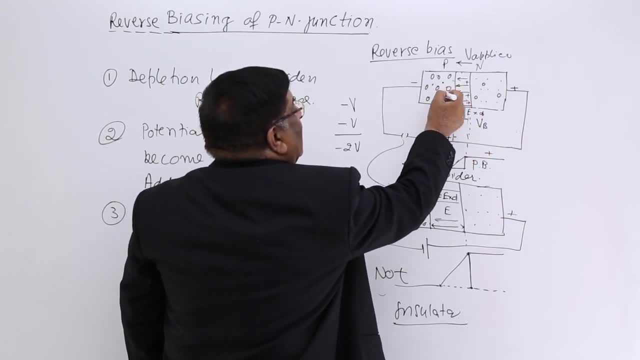 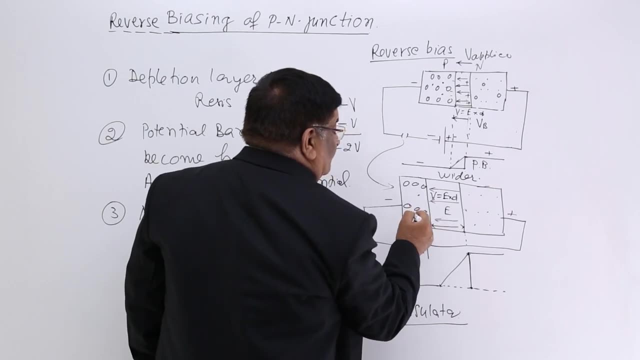 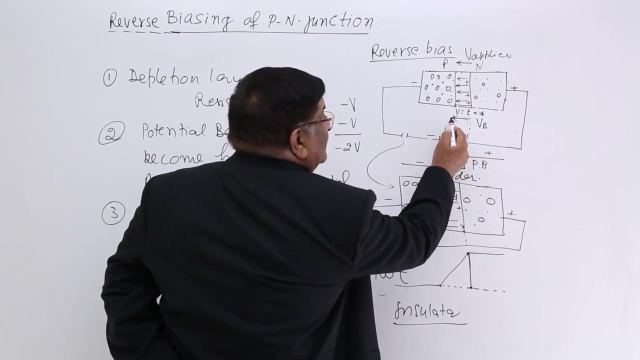 which are holes In this minority charge carriers are electrons. Now, this potential barrier which has increased so much, What is its effect on minority charge carriers? The direction of potential difference is plus to minus here, whether it is barrier potential or whether it is applied potential. 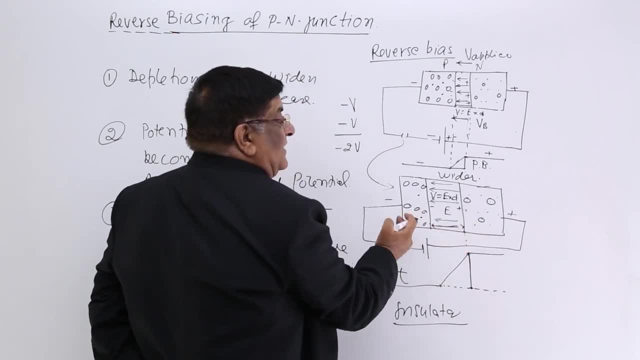 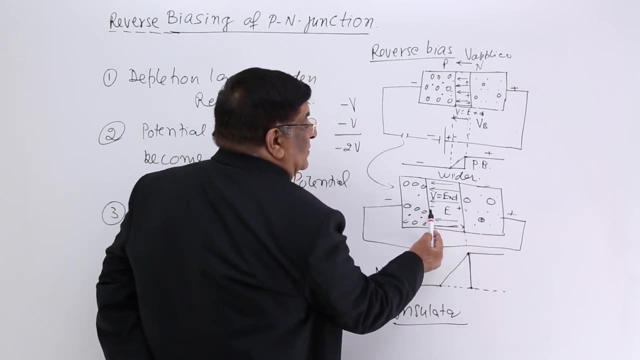 both are in this direction. That means the total potential is in this direction and this positive charge very happily it will go from higher potential to lower, from plus to minus. So this goes very well here. Electrons always go against potential difference, so electrons will go towards this. 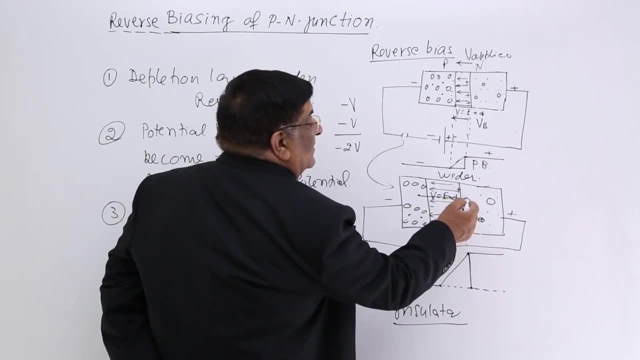 positive plate and electrons will move here, recombine with this. So when electron goes from here, another electron come from here. So this is a positive charge, This is a negative charge, This is a positive charge, This is a positive charge. When this hole goes here, another hole come from here. So what we see? 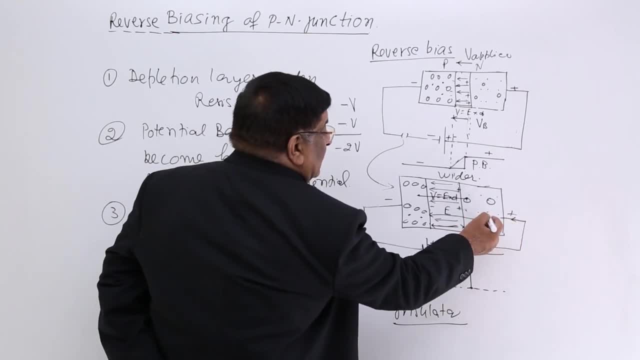 the positive charges from battery keep going here, Keep coming here. How These positive charges, these three holes have gone here. So in place of these three, there is a pull and three positive charges come here. Then again three go, again. three come from here. 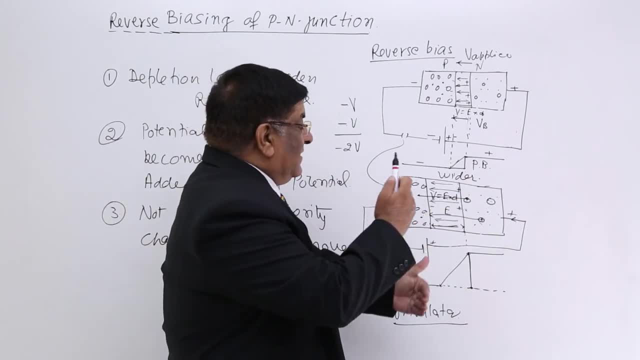 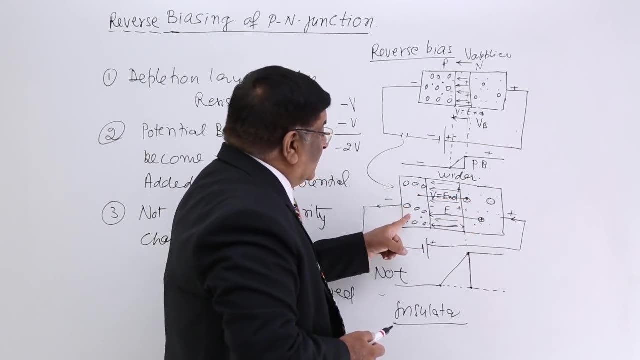 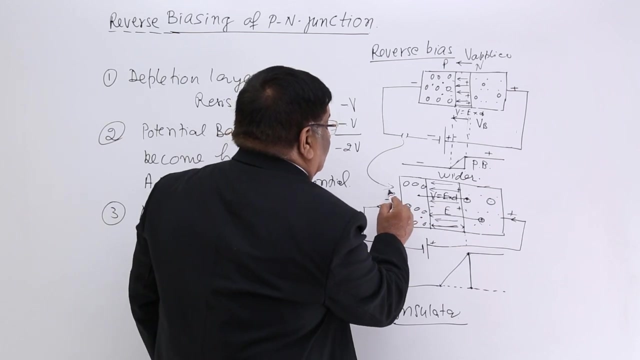 Again three go, Then again three come from here. This you can understand the other way. These three electrons go and neutralise them, So there is a shortage of three electrons. this becomes little positive and pull three electrons from here. Those three electrons, these three electrons. 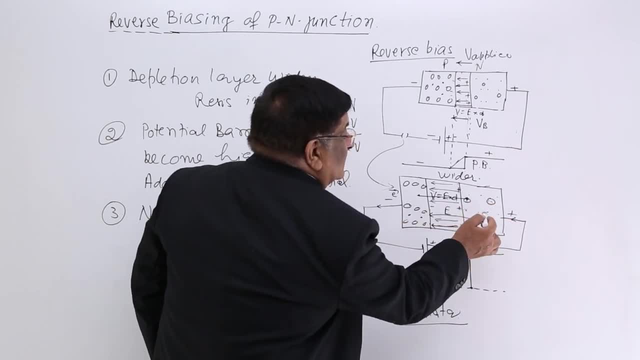 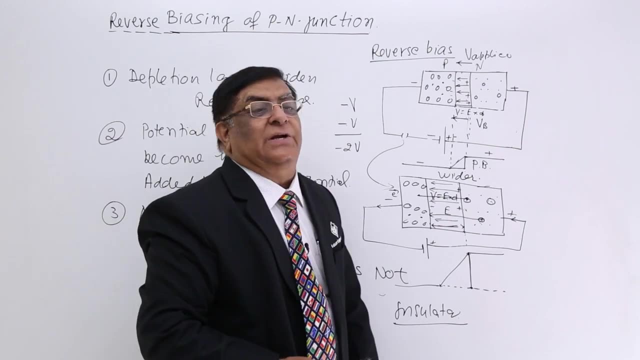 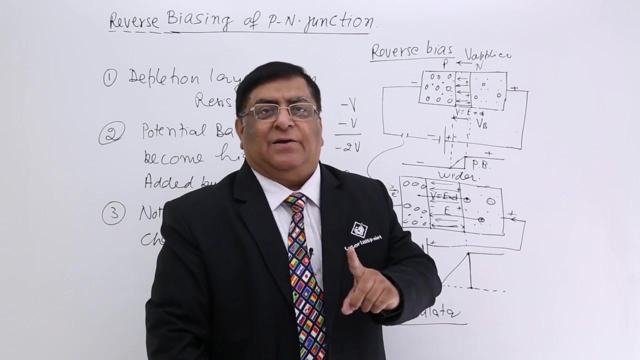 they have gone here. So these three again go to this, this three again go to this, and a current go in this direction, current goes in this direction. but how much is that current? This current continue. How much is that current? This current may be equivalent to 1 charge. 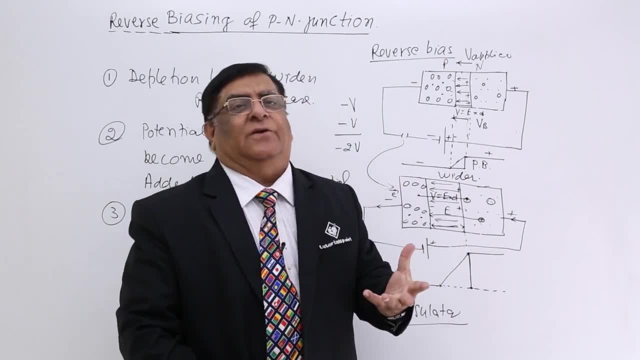 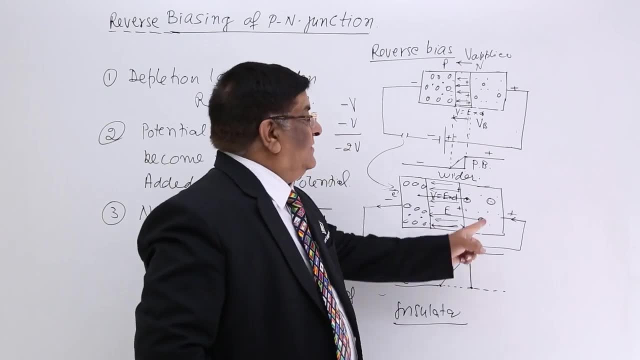 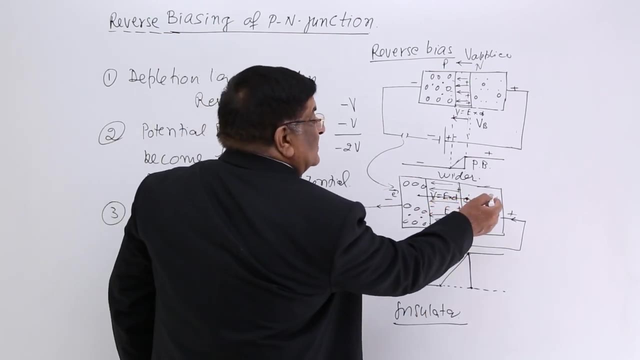 or 2 charge or 3 charge, depending how many flow, but cannot be 4 charges current, 5 charges current. Why? Because this is the maximum number. And when it comes to majority charge current, how many majority charge carriers are there? Answer: thousands, So majority. 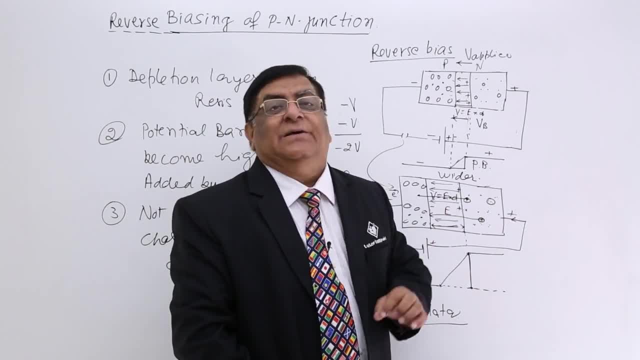 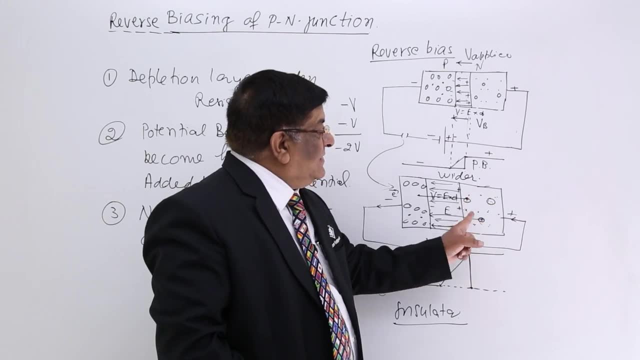 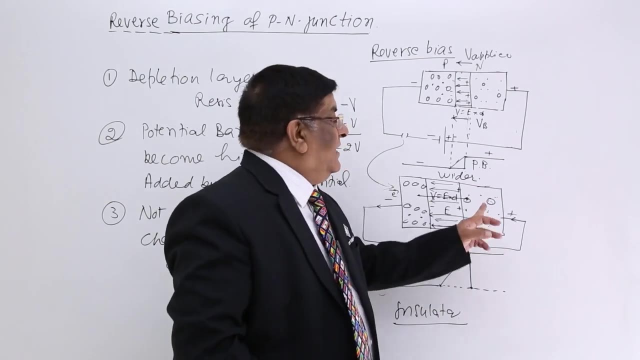 charge carrier. when we flow in forward, biasing, that is in thousands of microamperes, but when we flow, reverse this. the current, due to this minority charge carriers. this is a very small current because their total number is less, the charge carrier is less and the 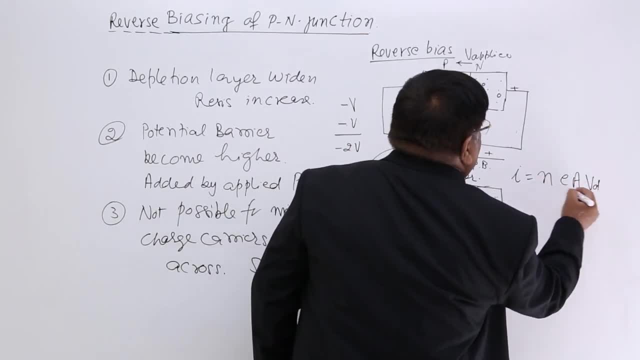 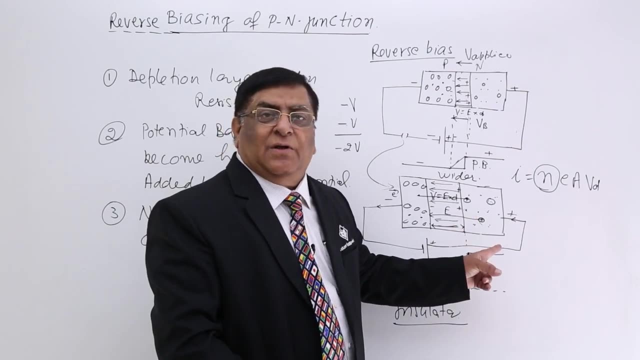 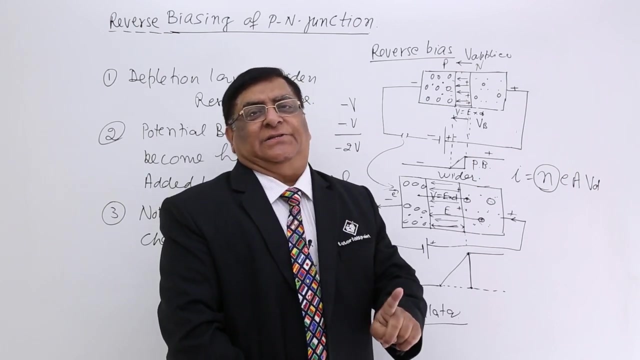 current is made by n charge carriers. So that is the number of charge carriers. So the current is E, A, V, D. This is number of charge carriers, and here number of charge carriers are very small. Now this current, which current in reverse biasing, made by minority charge carriers. This current is known as: 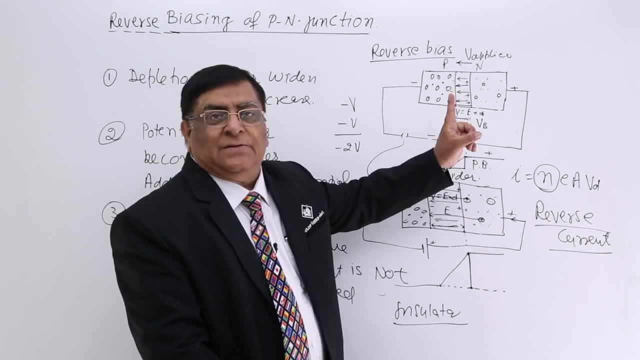 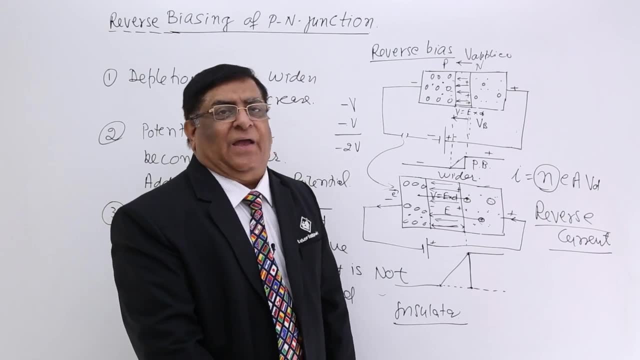 reverse current. In reverse bias the majority charge carrier current is not allowed. That is the main current. But at the same time a very small current is made by the majority charge carriers And this is the number of charge carriers. So the number of charge. 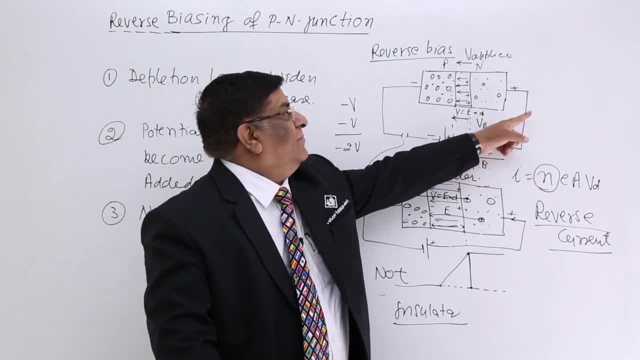 carriers made by minority charge carriers is constant. Well, recall that emerging in reverse and preceding current, current going down. There are most of them, A強ierten characteristic of reverse bias � formidable point loving and threw. So, a very small current keep on flowing from plus to minus. A very small current keeps 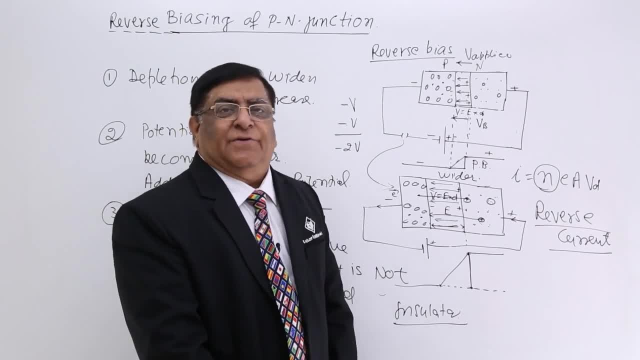 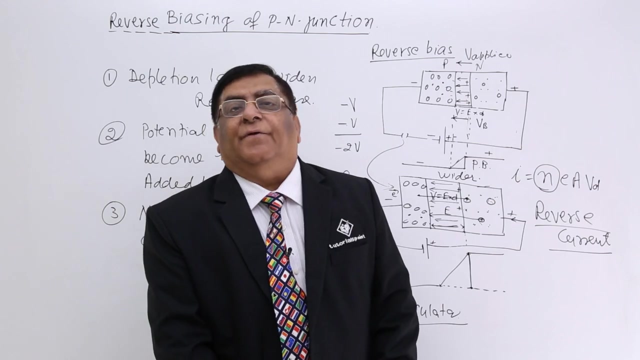 on flowing due to minority charge carriers. This is in reverse biasing due minority charge carriers and we named it reverse current. So a reverse current keeps on flowing in the reverse biasing. So this is reverse biasing results. So for normal use, while 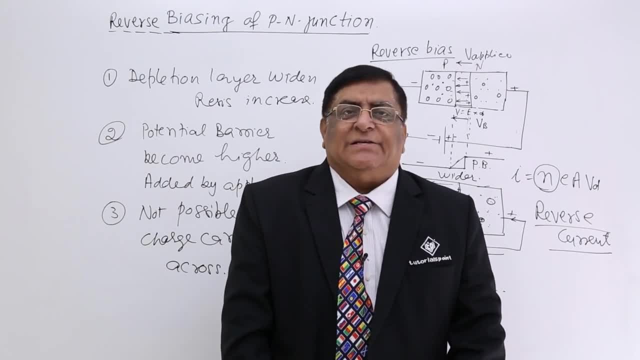 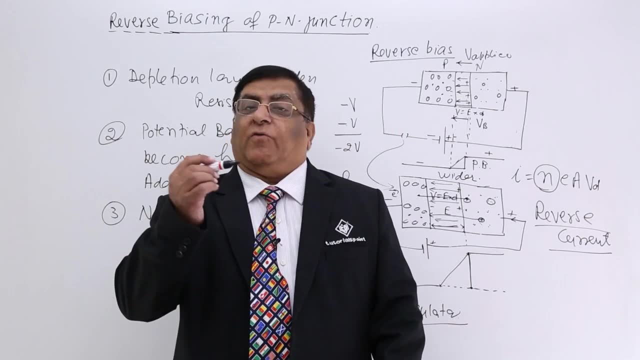 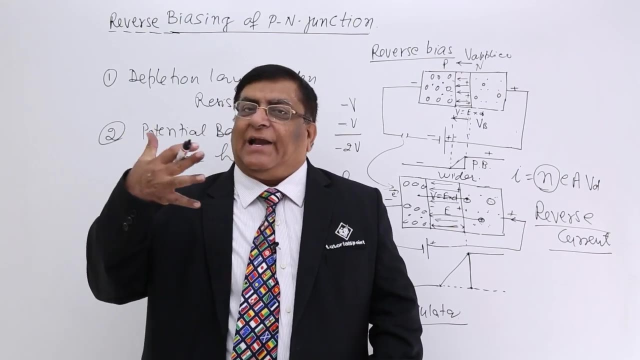 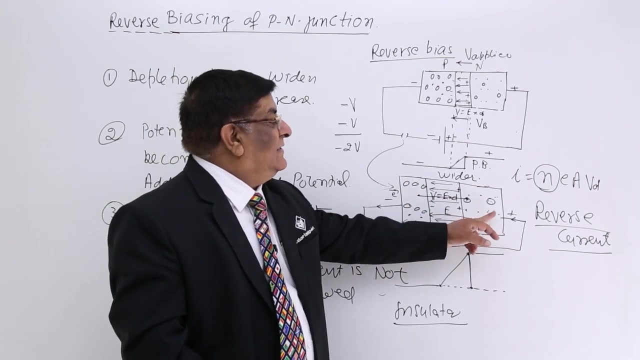 this current will flow in. And then, when the current is in lower color, is that picolour 작은, What we say? This reverse biasing current is very, very small. Say 1 upon 1000 of the forward bias current. So for us it is no current In forward biasing, there is a current of 1000 milli amperes In reverse biasing. all these are blocked and there is no current due to majority of charges.